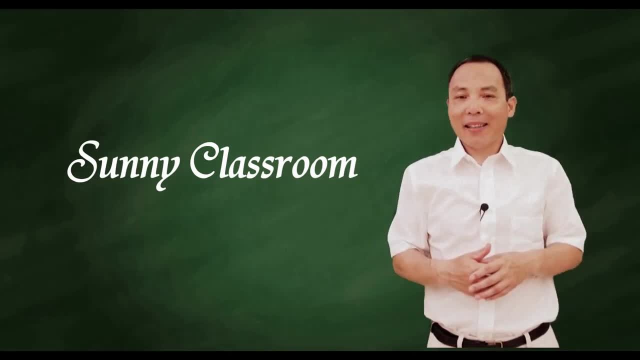 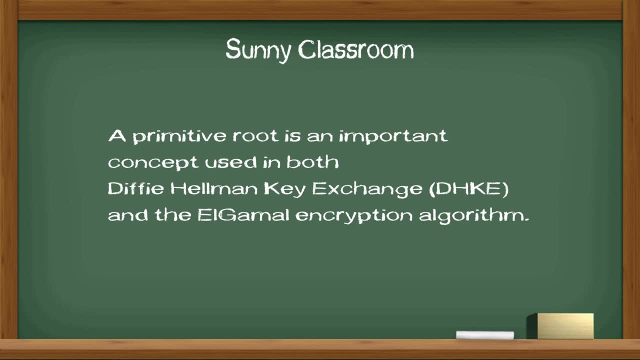 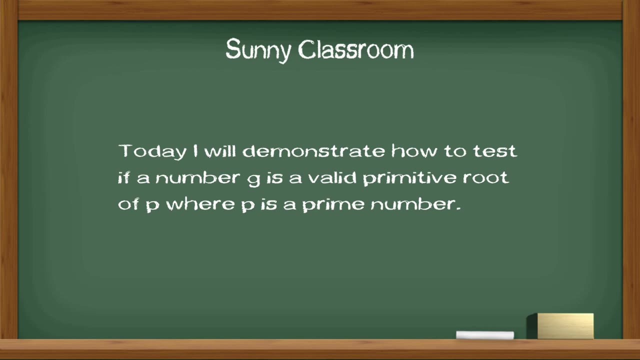 Hello, and this is Sunny. Welcome back. A predictive route is an important concept used in both Diffie-Hellman Key Exchange and Agamal encryption algorithm. Today I will demonstrate how to test if a number G is a valid predictive route to P, where P is a prime number. 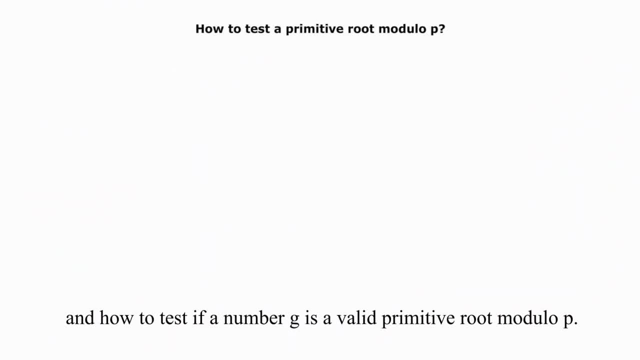 And how to test if a number G is a valid primitive route modular P. The fact that G is a primitive route, modular P must satisfy two conditions. One, G bigger than 1 but less than P. Two, the modular results must be distinct. 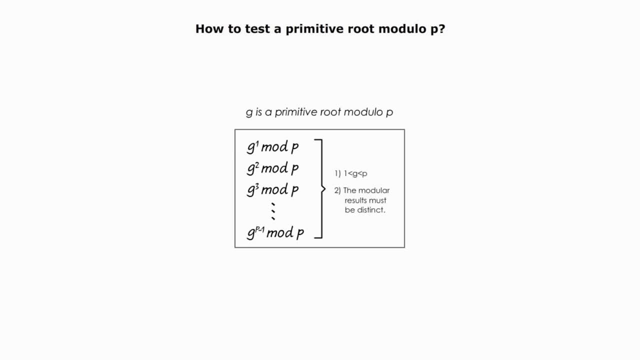 The first condition is that G is a valid predictive route to P. The second condition will bring many questions. First you need to understand the modular operation is simply to get the remainder. Thus, all these remainders must be unique And there is no duplicate. 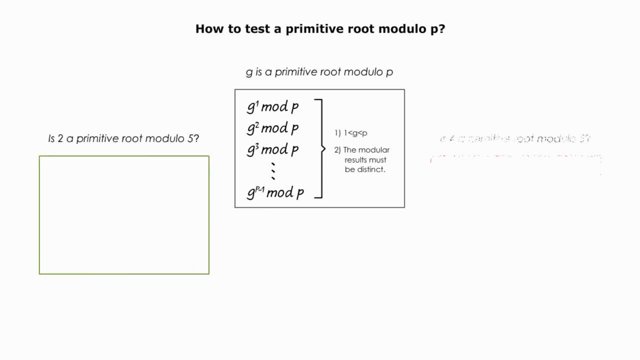 Let me use very small numbers to understand the number G. Suppose P is 5, very small number is a prime number is 5.. Let me test if 2 is a primitive route, modular 5.. 2 modular 5 is 2.. 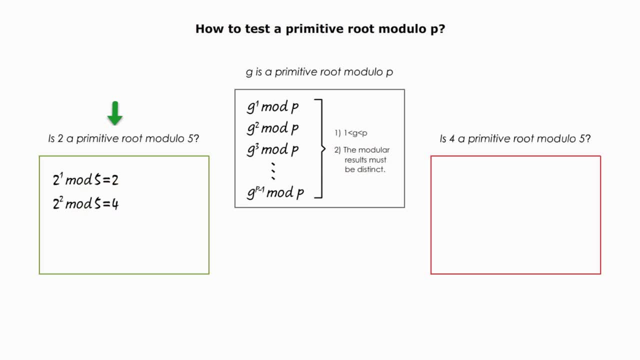 Thus, the remainder is 2.. 2 to the second power is 4.. 4. modular 5 is 4.. 2 to the third power is 8.. Modular 5 is 3.. 2 to the fourth power is 16.. 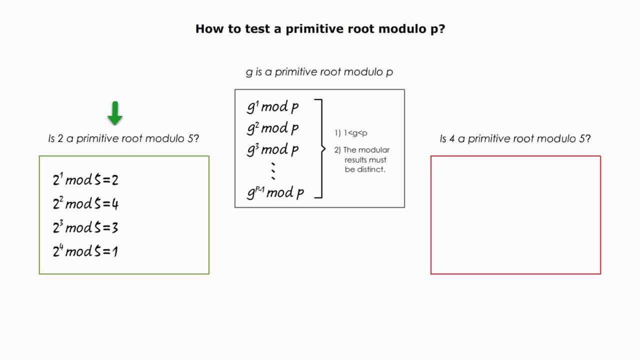 And 16. modular 5 is 1.. So it simply is just to get the remainder And you can see even very small numbers are tedious, But you get the idea. Let me test. 2 is a primitive route, modular 5.. 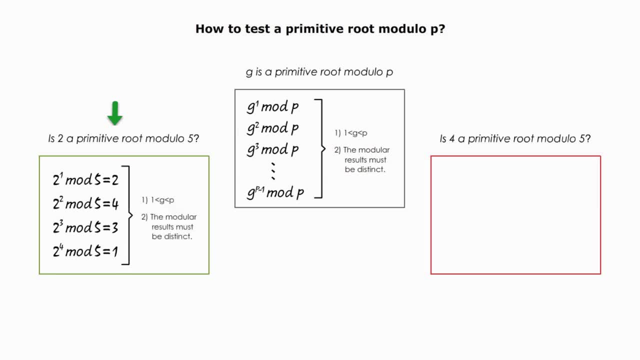 2, bigger than 1, less than 5.. The first condition is met. It's OK. The second condition: the modular results 1, 2,, 3, 4, are distinct. There's no duplicate. 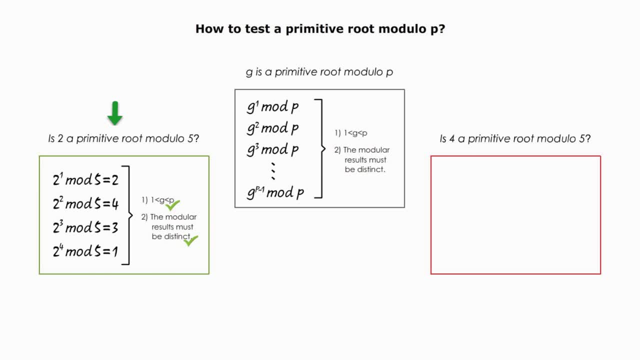 Thus the second condition is met, Both conditions are met And we can say: 2 is a primitive route, modular 5.. Let me test if 4 is a primitive route, modular 5.. Let me test if 4 is a primitive route, modular 5.. 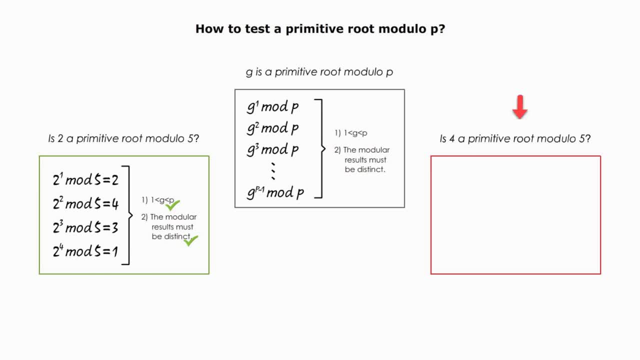 4 modular 5 is 4.. 4 to the second power is 16. And 16 modular 5 is 1.. 4 to the third power is 64. And 64 modular 5 is 4.. At this point we can say 4 is a primitive route, modular 5.. 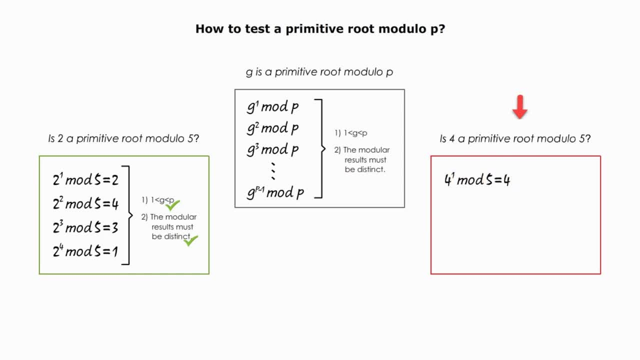 4 to the second power is 16.. And 16 modular 5 is 1.. 4 to the third power is 64. And 64 modular 5 is 4.. 4 to the third power is 64. And 64 modular 5 is 4.. 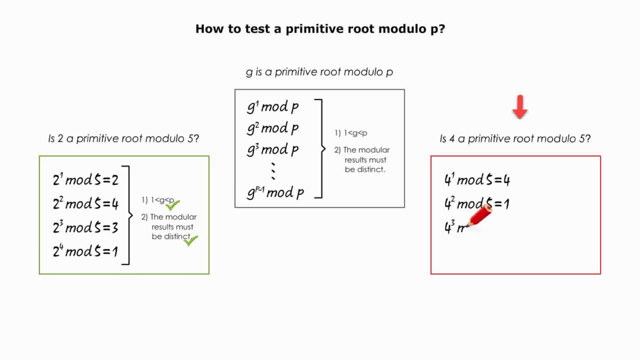 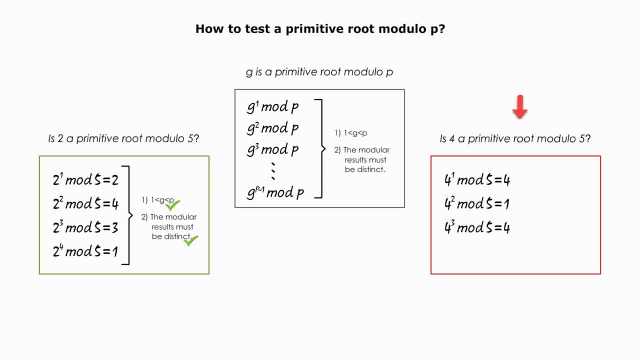 And 64 modular 5 is 4.. And 64 modular 5 is 4.. and 64 modulo 5 is 4.. At this point we can see there's two duplicate results: 4.. If we continue 4 to the fourth, power is 256, and 256 modulo 5 is 1.. Again, the result is the same as the second. 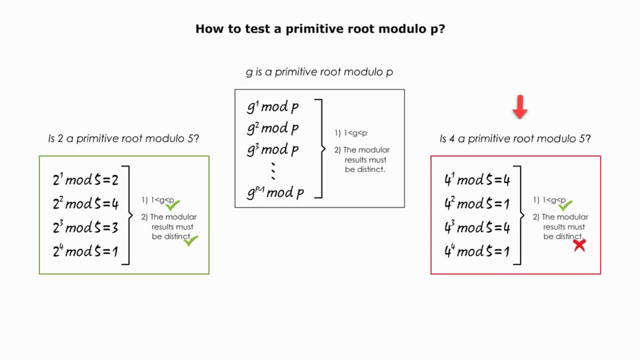 one. The first condition is good, but the second condition is not good. Thus 4 is not a primitive root of modulo 5.. You can imagine if p is a very, very large prime number. there would be a loss- loss of primitive roots. But computers can handle calculations. I hope this video is. 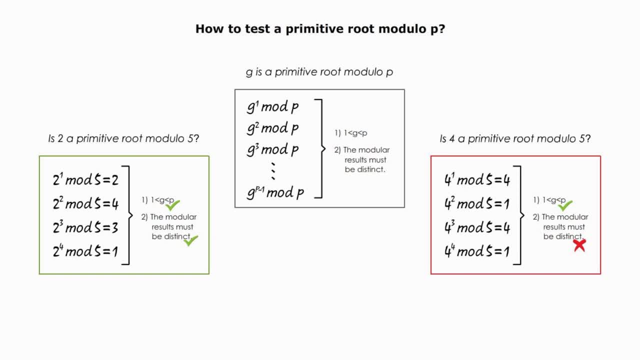 helpful. Thank you very much and see you next time. 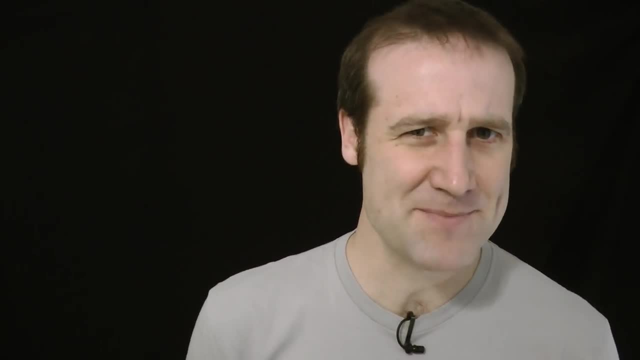 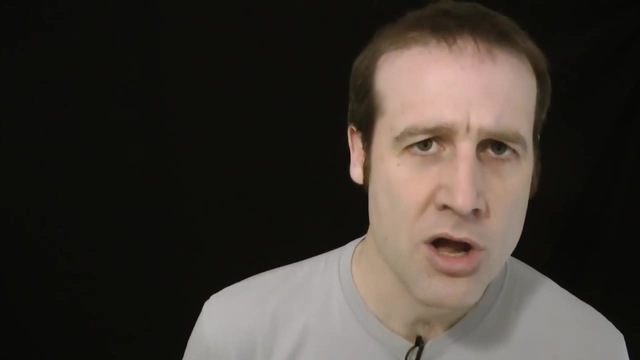 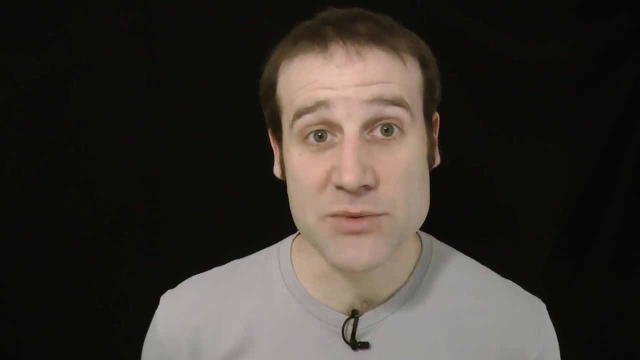 2016 is a leap year and that makes me very excited. as much as I mourn the loss of February, no longer being an integer number of weeks Long, I still love leap years because, frankly, calendar drift is a serious issue. In 1627, during the Anglo-French war, the English army invaded. 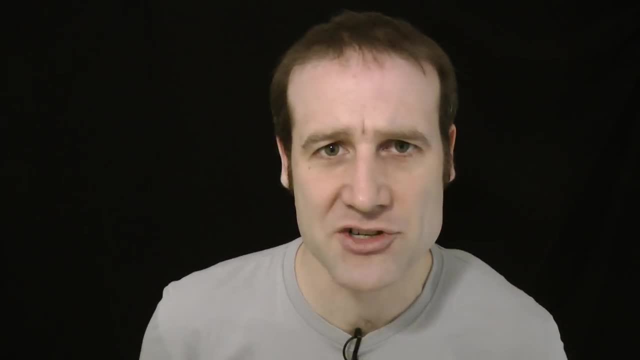 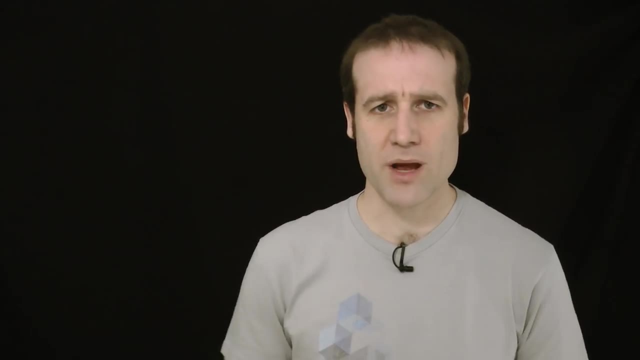 one country was the 22nd of July for the other country. It was all very confusing. At the very least, both countries agreed it was a Thursday. Calendars were born way back in pre-history as a way to keep track of the seasons and to this day we use them for pretty much the same purpose.